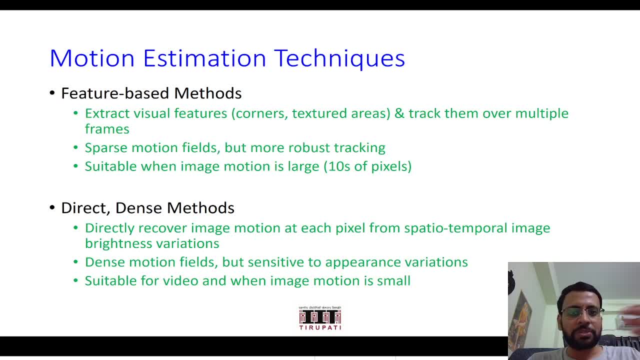 the image motion of the order of tens of pixels. The other category is direct-dense methods, where each and every pixel, you would be computing the. what are the motion vectors there? what are the velocity vectors in the x and y directions? And this is what. 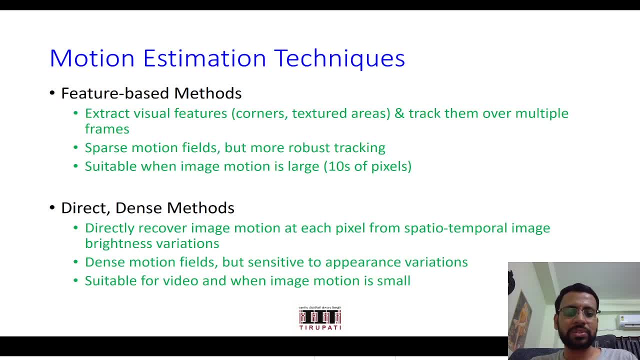 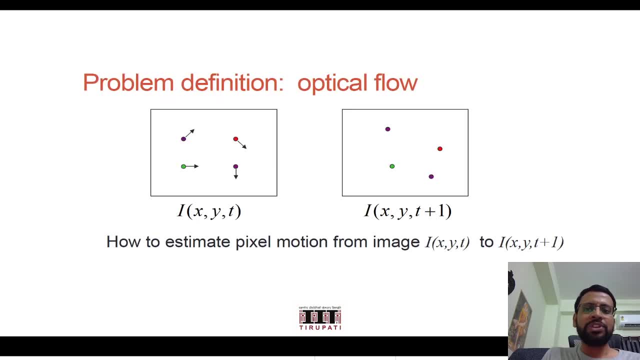 we will be discussing in this lecture and next few lectures And more specifically, we will be talking about optical flow methods. Well, to get some intuition about the optical flow methods, this slide helps you. So assume that you have three points in three different colors. 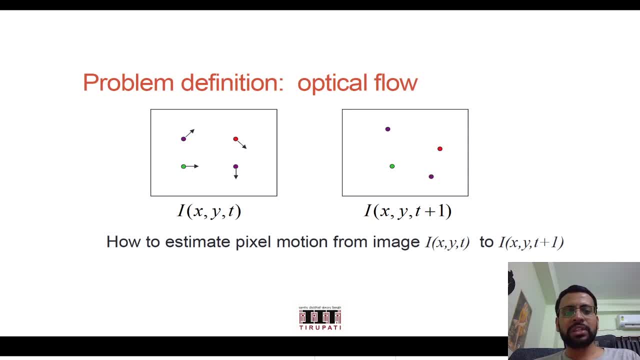 as shown on the left-hand side of this image and the subsequent. assume that they are moving and you have next frame at the next time instance. what you have is initially- let's call it as I- of x, y, t. next time frame you have at t plus one. 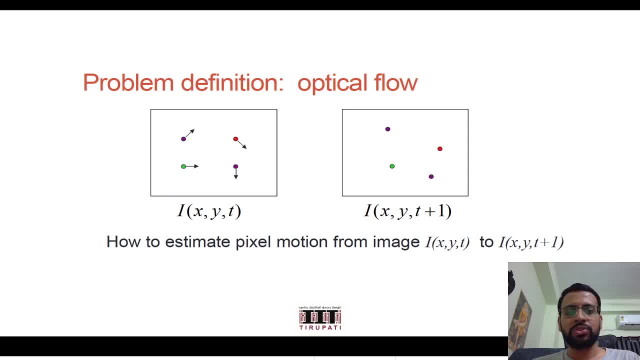 time frame, you have the second image. The goal is now to understand where the second, where these pixels with different colors have moved So well. some pixels could have the same color, like, for example, those on the diagonal pixels, both diagonal element in the diagonal, whichever are there. 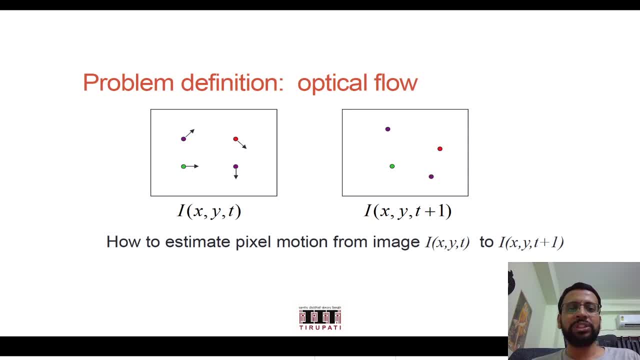 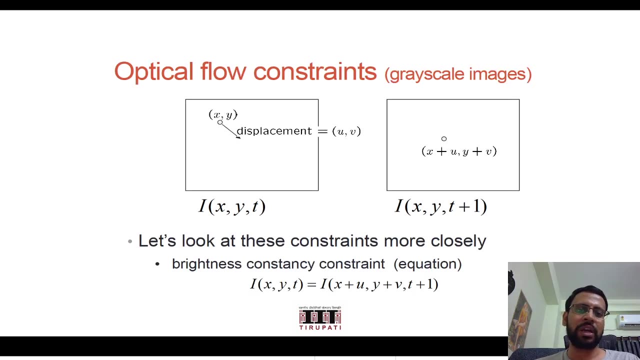 So what optical flow does is it looks in its surroundings and figures out the one with the same color and then from that it estimates as the value of x and y. This we have seen in terms of colors, but what we, in grayscale images, would be looking for, 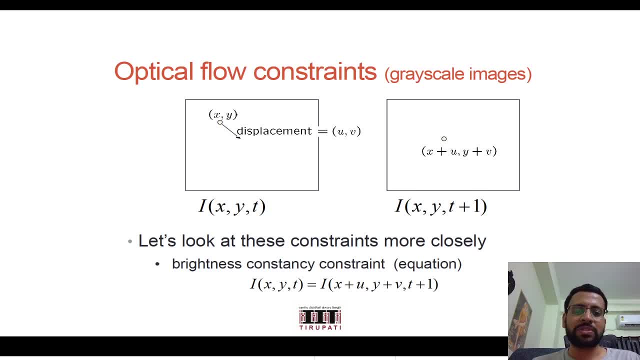 is pixels with the same brightness value. Assume you have a pixel location at x- small x, small y in the first frame as a specific intensity here and what you assume, the constraint as it says: brightness constancy constraint. So our assumption: 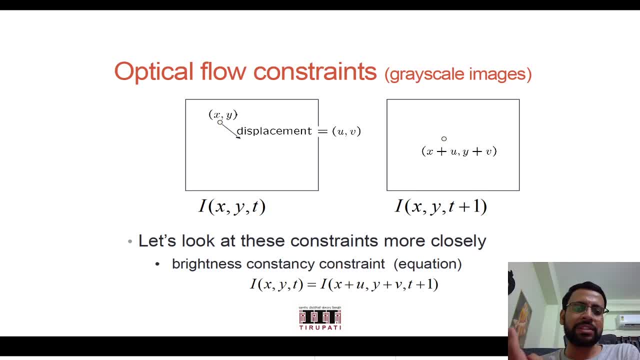 here is: the brightness of the pixels would remain same despite a movement. That's the assumption. So the second frame, which is a slight movement from the first, one of the objects within that scene, so what you would look for there is you will be looking for a. 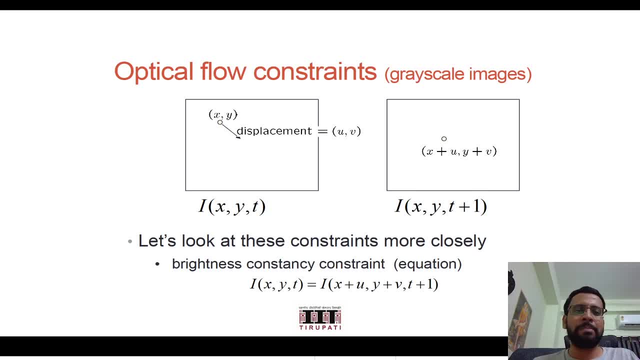 pixel that has in its surroundings that has the same brightness constant. So, for example, that's what the last equation has been given there I have- xyt is equal to. we assume that it has moved by a small value, u, in the x direction and 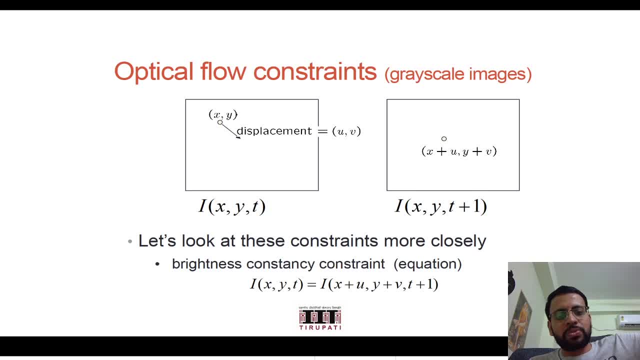 a small value of v in the y direction. So you would find out now a pixel which could be at a location x plus u and y plus v, and this u and v being the values to be find out at the end of your process. 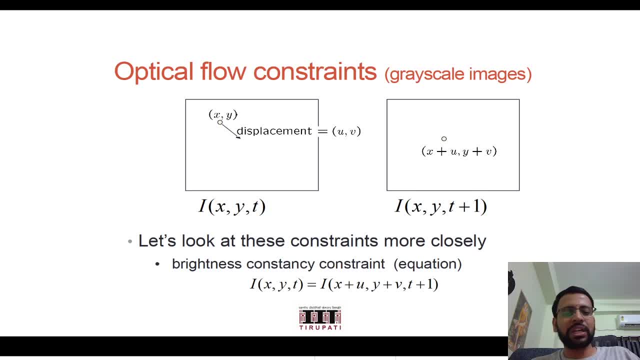 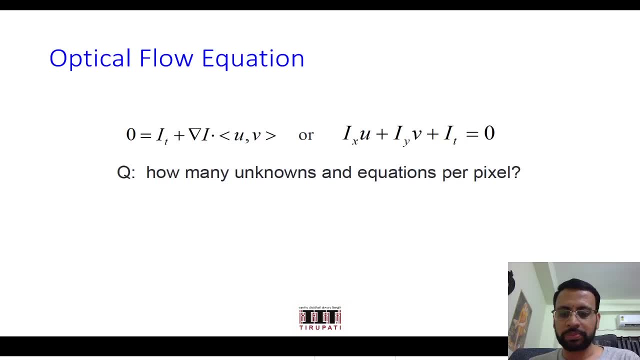 And it is in the t plus 1th frame. So that's all you are going to do. Let's now derive the basic equation for this optical flow. So let me move on to a different scene here in my OBS studio. 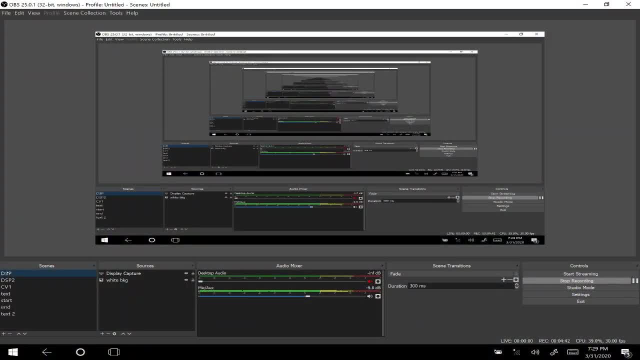 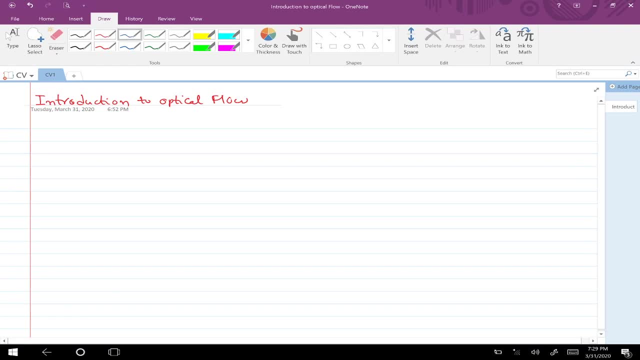 This should solve the purpose. So let me do the workout here in a notebook here. So what we are going to do is, in the first image, whichever is there pixel is there at x comma y. location at the tth frame. Now you would like to find out. 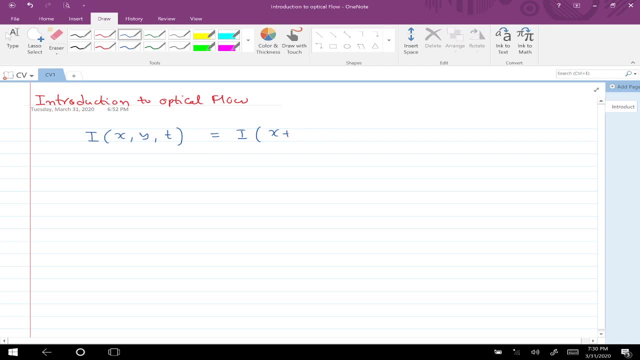 a corresponding pixel which has same intensity. For that you can move a small value of u in the x direction, v in the y direction, and this you are looking at, the t plus 1th frame. In an ideal case, this would mean that what your u and v should be such: 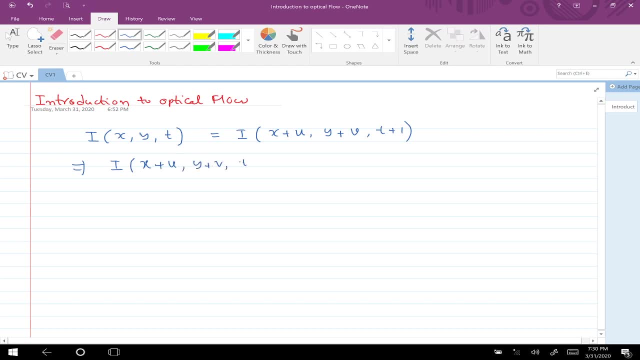 a way that y plus v, comma, t plus 1, this minus i of x, y, t should be 0.. Now assume that u and v are small, very small. So again in the regular process you go to, your savior is tyler series expansion. 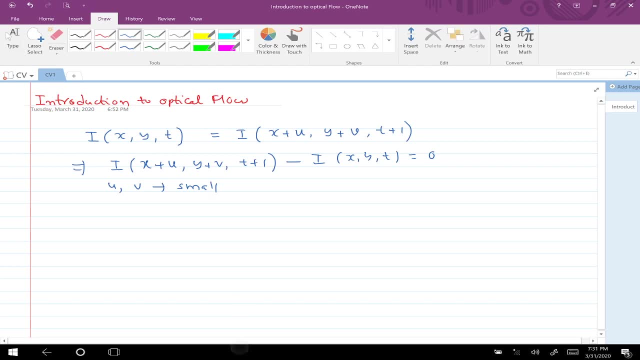 You do a tyler series expansion for the first term with respect to, for example, being x comma y comma t being your reference, plus dou i by dou x. I am dropping writing of x, y comma t here for just the briefness and of course in the x you have 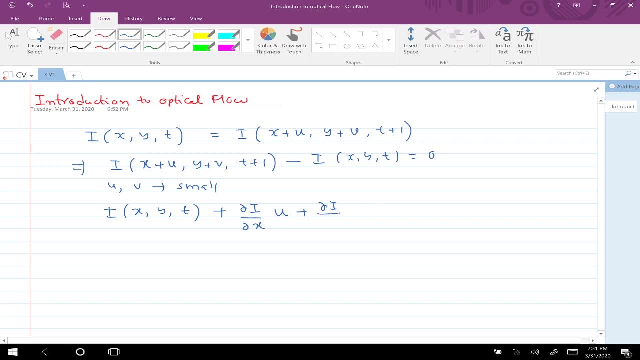 u plus dou i by dou y. in there you are assuming it v and for t. what we would do is you consider t plus 1 and t plus t, so then I could write it as dou i by dou t of t plus 1 minus t. 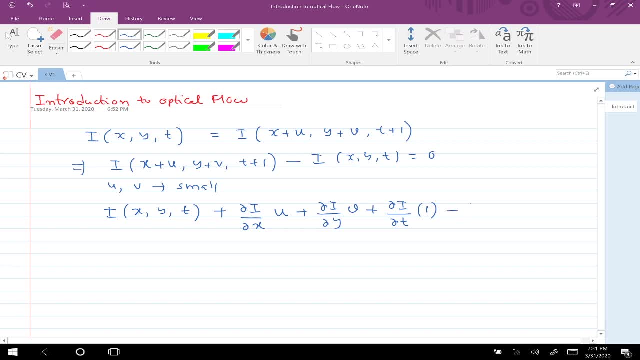 so that is 1.. This is the first term minus i of x, y, t equal to 0 and, of course, ignoring higher order, you are also ignoring second order terms. ok, ignore second order, all the second order terms. so then that is what would happen, ok. 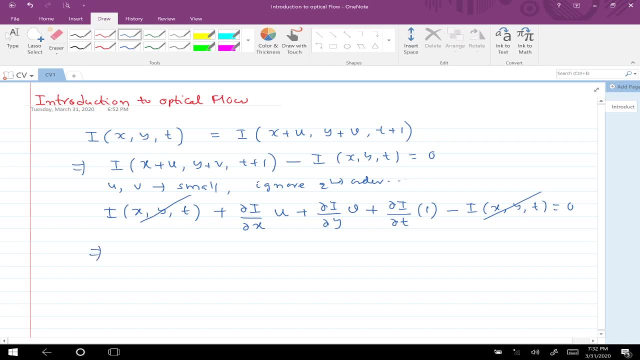 these two would cancel out. it would give you now a dou i by dou x into u, plus dou i by dou y into v, plus dou i by dou t equals to 0.. Let us again use for compactness. let i subscript x would give you. 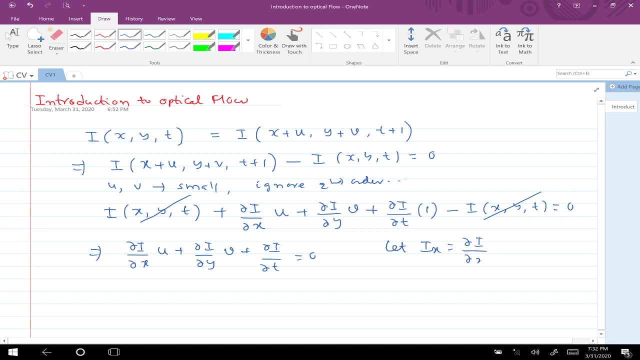 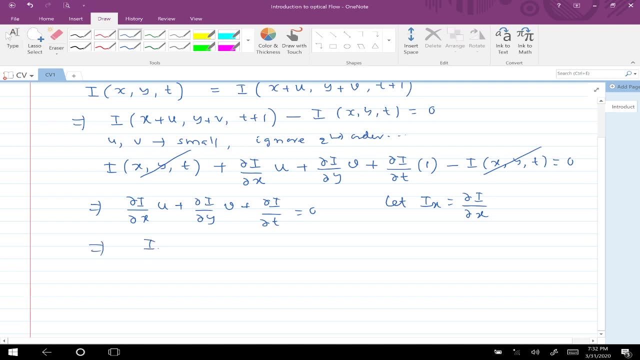 dou i by dou x. So same case with the y and t as well. so then i could write this equation as i subscript x into u plus i subscript y into v is equal to minus i t. ok, if you want, this is the equation for optical flow. 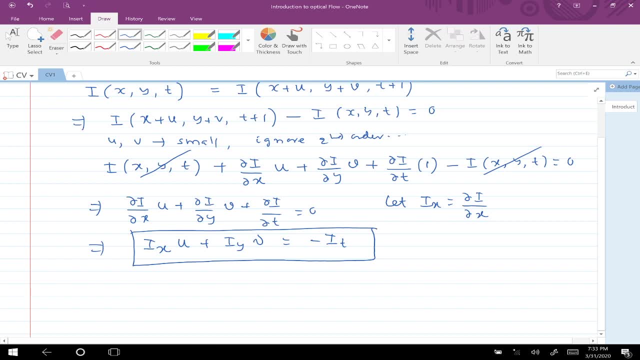 right, assuming brightness constant by imposing a brightness constancy constraint. this is the result of the brightness constancy constraint. you are assuming that brightness is constant, so that is why you are making that equal to 0. ok, you could in fact write it in vector form as well. 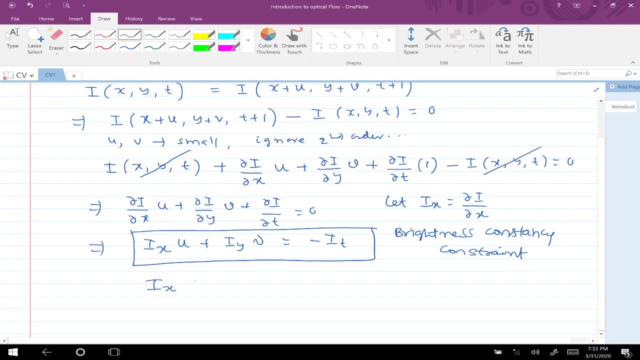 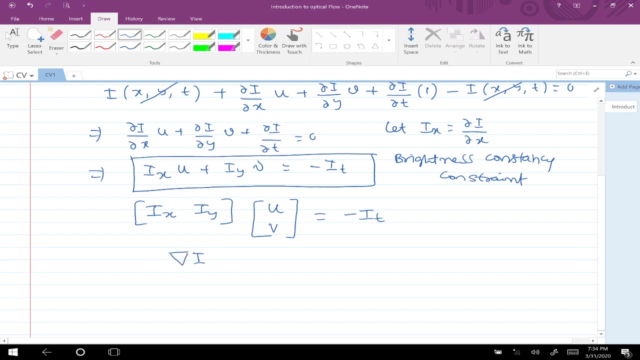 if you want, for example, i could write it as: i, x, i, y multiplied with u- v would give me minus i t. i could also write it as this: as gradient of i and its dot product with u comma v would give me minus i t. you would see shortly. 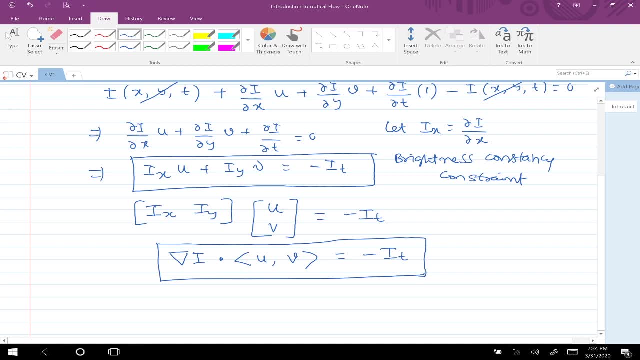 for a geometrical interpretation of optical flow solution. this second representation would be handy for us. another point to note here is: how many variables are there? what are the variables here that we need to find out at each pixel? the displacement in the x direction and the displacement. 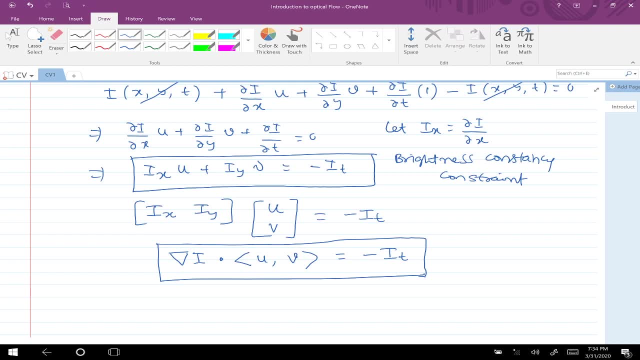 in the y direction. so u and v are the variables to be computed. and how many equations are there? both equations are same, except that we have written it in a slightly different form. so you have a single equation here. it means you have multiple possible solutions if you impose. 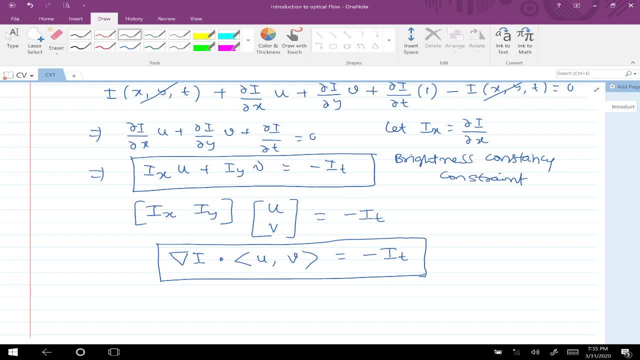 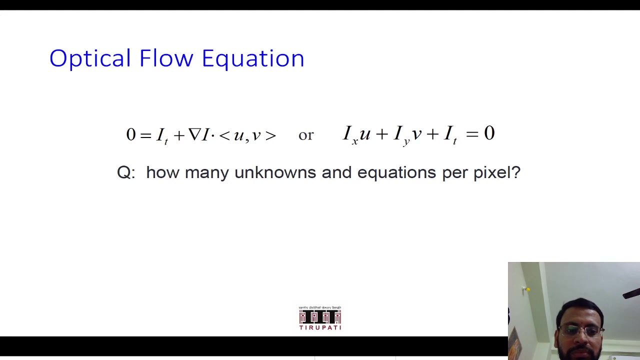 just the brightness constancy constraint at each pixel. if that is the only constraint that you are posing, it has multiple solutions. ok, yeah, with that again, let me come back to the slides mode. right, ok, now the same thing has been written here. i t is plus gradient. 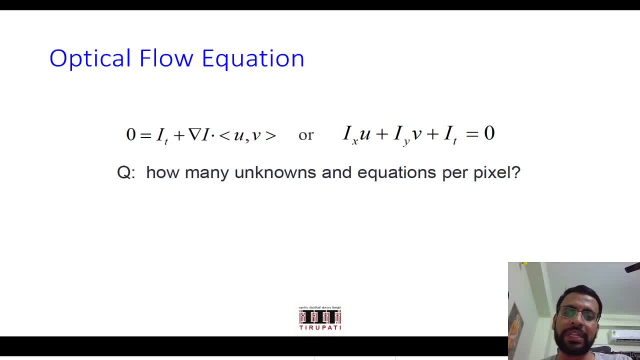 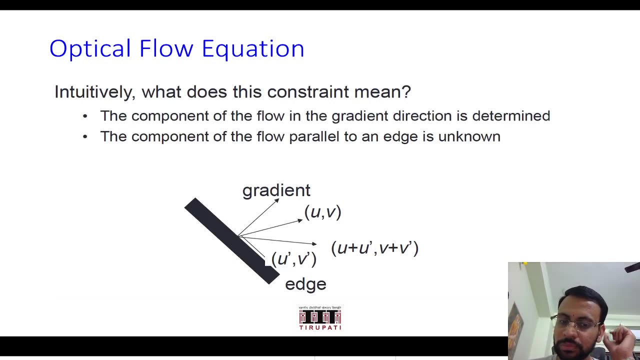 of i dot product with u comma v, that is equal to zero. or i subscript x times u plus i subscript y times v plus i t, equal to zero. this question we answered. it has two unknowns and single equations, so multiple possible solutions are there. look at here, let us take a. 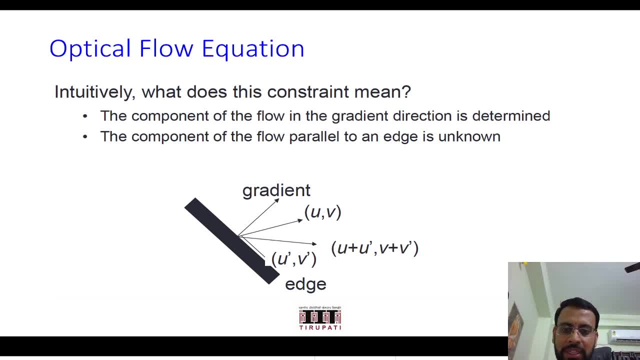 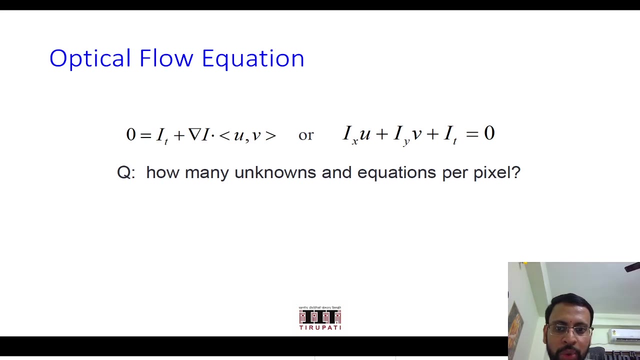 geometric representation of this in your image. assume that you have this being your. there is an edge in your image that you are looking at and gradient of it is there. so when you have gradient of i dot product with u comma v, that is what it is giving. ok. 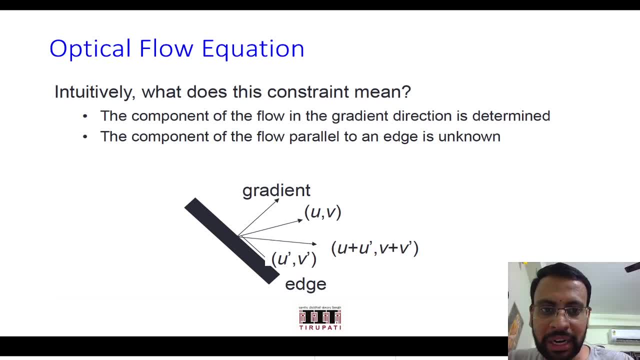 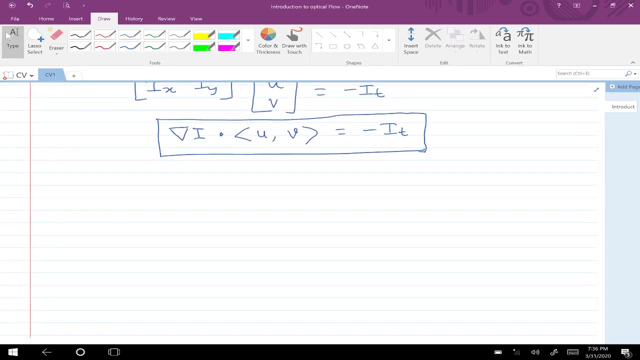 so let me maybe draw this again. maybe that drawing could help you to understand it easily, much easier. so let me again go back here. assume that i have a strong edge here. ok, there is a strong edge here. this is all fill it with color, so you have a. 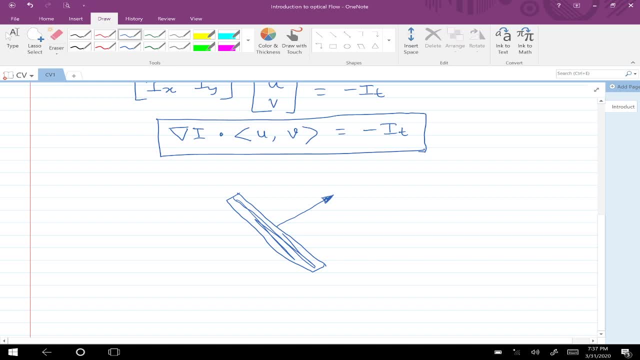 this is here the gradient at that point. this being your gradient, i ok now. the left hand side of the above equation is inner product of u and v. that is what you have there. so that means any it value. you know it. you see here. suppose this is my. 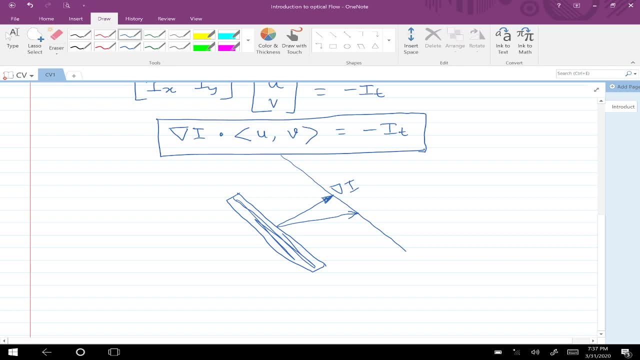 u and v is giving me this value, for example. that inner product is same as. even if my u and v values are here, are here are in fact, on the other side also. ok, so all these things would give you the same inner product when you do a dot. 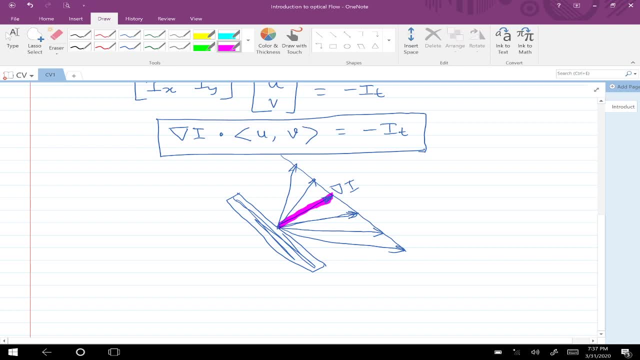 inner product with gradient of i, all these values of u and v, this- let us call it u1, v1, ok, call it as u2, v2, and so on, all of them would give you the same inner product, which could be equivalent to, let us say, the: 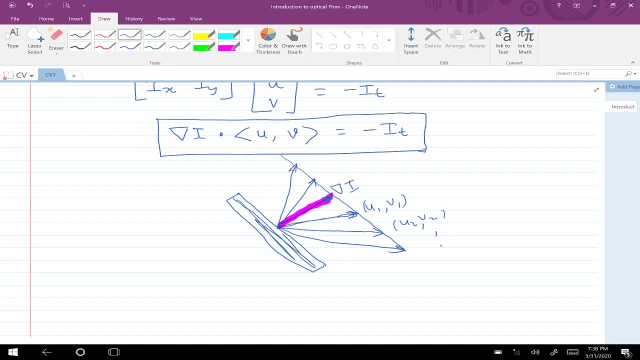 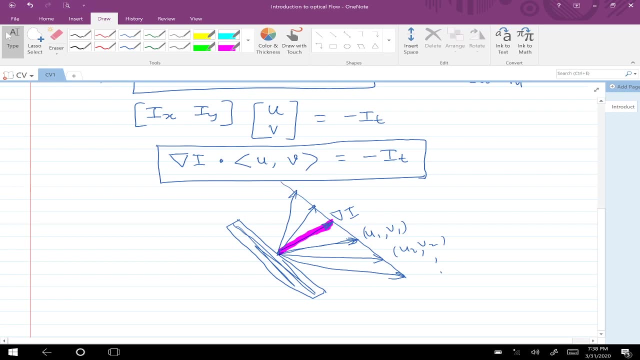 it that you are looking at. so this is another way of see. one way we had looked at is there are two unknowns and one equation presenting in multiple solutions. another way to look at it geometrically is: you have in the image. you have an edge here. 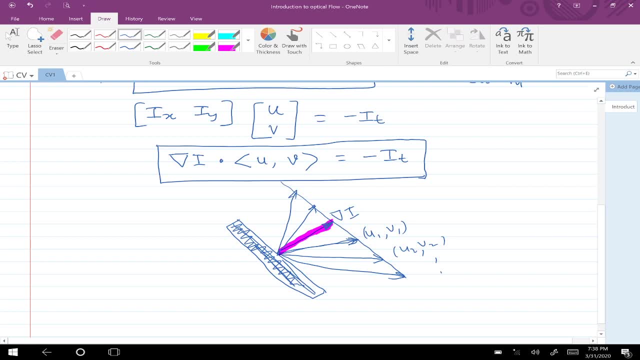 gradient perpendicular to it. on the left hand side you have, for example: it is nothing but i x comma y of t plus 1 minus i of x, y, t. that is a fixed one, very given image. you get it fixed. so, right hand side, you know the value. 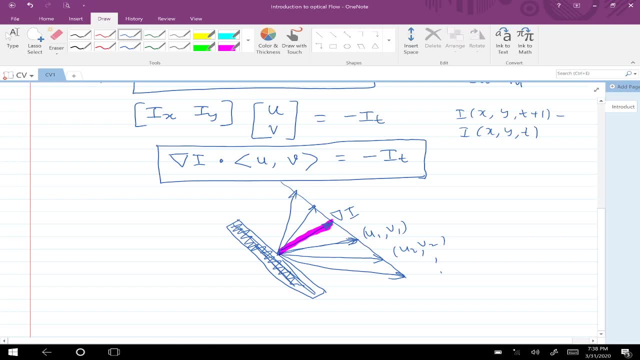 so suppose that is the value, we are fixing it so you get that same value for different u because you are taking only one of the components of it right, which is perpendicular component to the gradient. is all that you are taking here, right? so there are multiple solutions here. 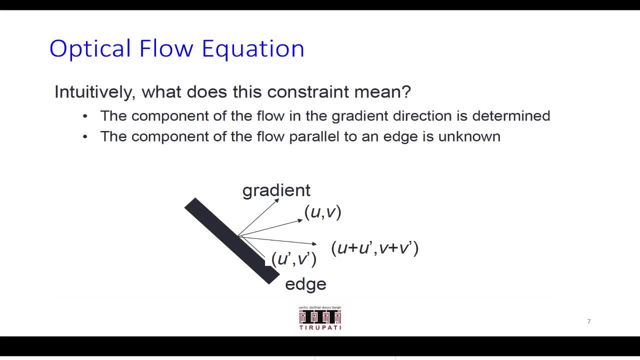 ok, let me go back to the mode here. so this is what the component of the flow in the gradient direction is determined. ok, that is what we are taking. component of the flow in the gradient direction is what we are taking and the component of the flow parallel to the edge is. 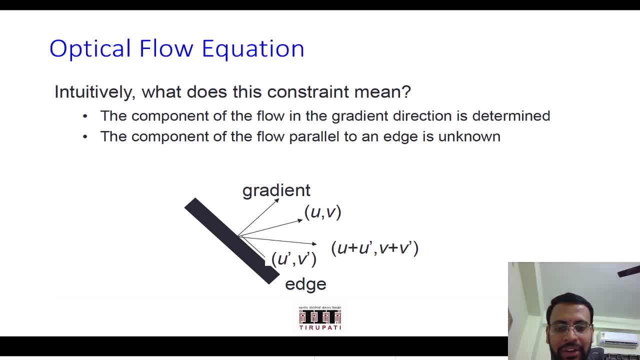 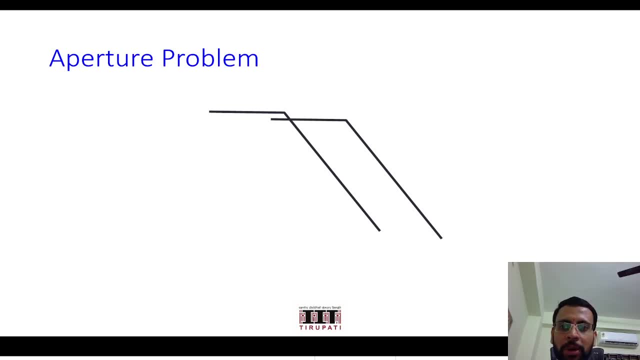 unknown. you could have any parallel components, would have any of those things the way we have plotted- and this is not a new problem, this is an aperture problem. hope you still remember where we have discussed about this aperture problem. we discussed it in case of corner detection, if you recollect. 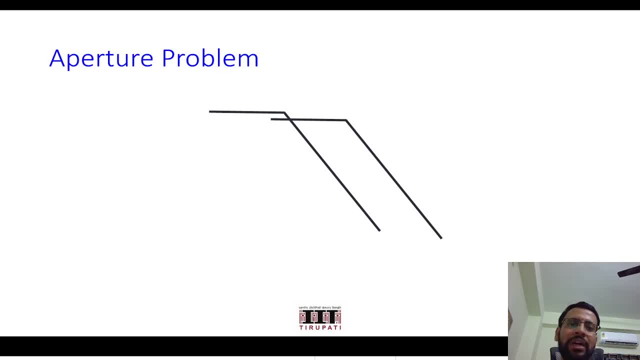 harris corner detector. we have seen there, for example, in a uniform region you have an aperture problem, you do not really know the corresponding point, identical point, exactly, and also while you are moving across an edge to find out even not just detection but finding out the correspondence. 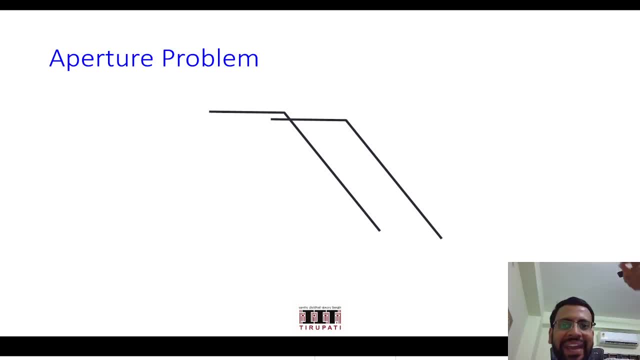 there will be multiple correspondences while you are moving across an edge where there is no textural difference or where there is no corner as such. right same problem you again face here when it comes to optical flow as well. again a quick an illustration of it. for example, if you 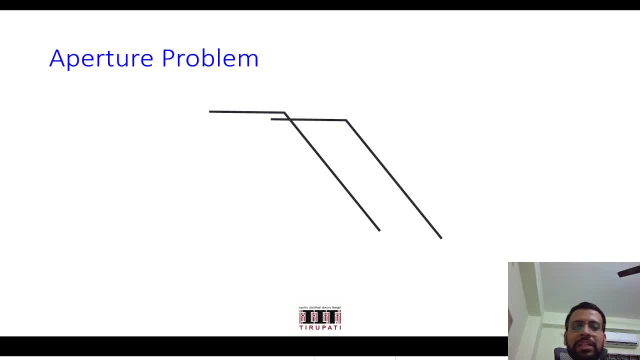 have something like this: okay, your object has the first one is your assume that your eye of x y t and another is x y t plus one you could see there is. you could see here which point maps to what when you have the big picture but optical. 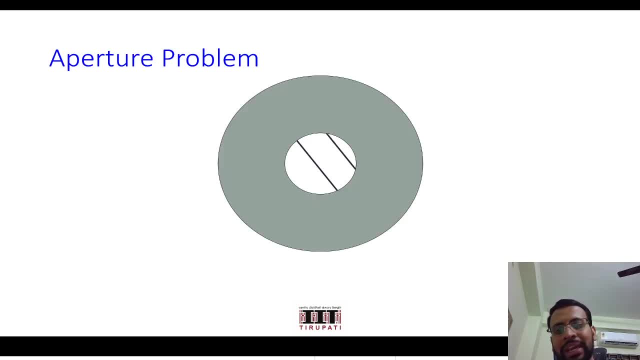 flow you are looking at locally. assume that when you are looking at a very small neighborhood there, you do not know really which point corresponds to what and you know only in the parallel direction. you have no clue there. okay, another depiction of this is this: suppose you only see in a very 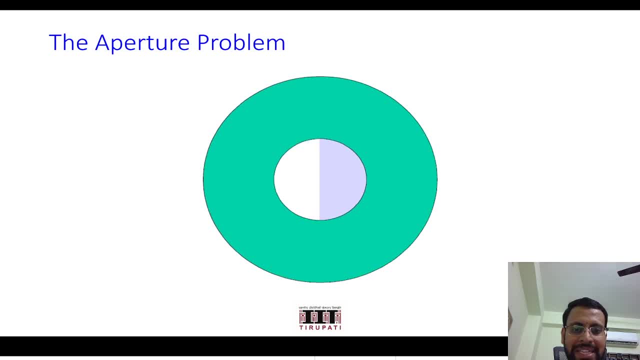 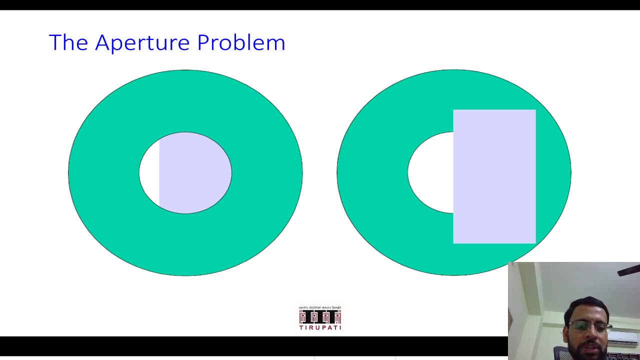 local region. okay, this appears as if the points have moved. even for us, visually looks like the points have moved parallely, but what could be the case here is this could be the actual one- that getting hindered from you is what has been shown now on the right side. that might. 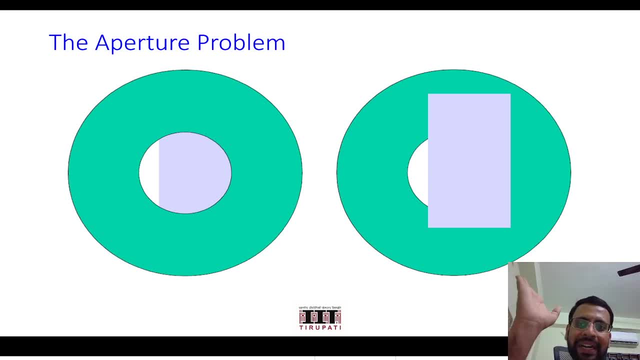 be moving in a diagonal top right diagonal. it might be moving, but that could never be inferred. all you could see is in the perpendicular direction, is all to the edge, is all that you could see there. but whatever is there in the parallel direction across the edge, you 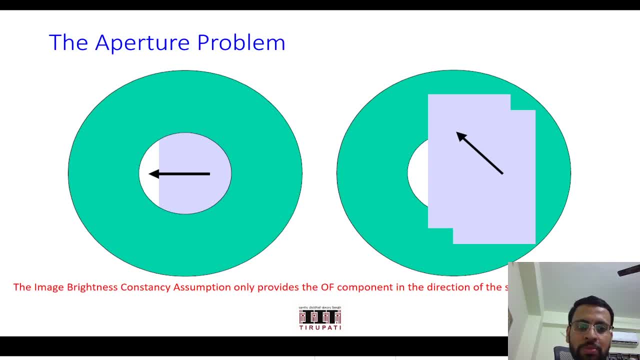 will not be able to infer so while it has moved in the perpendicular direction, what you could all say is the movement perpendicular to the edge, but you could never infer to the parallel, what is exactly the component? that same thing we have seen from the inner product as well. 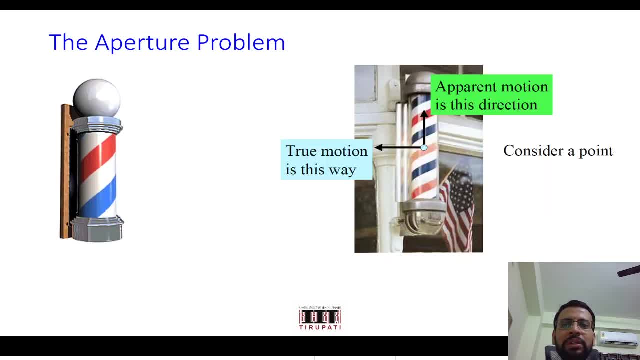 right. this is another example of this aperture problem. when you focus yourself in the local regions of those colors, all you would see there while moving, it looks like as if the colors are moving in. the apparent motion looks as if it is moving perpendicularly up, but when you see the bigger picture, 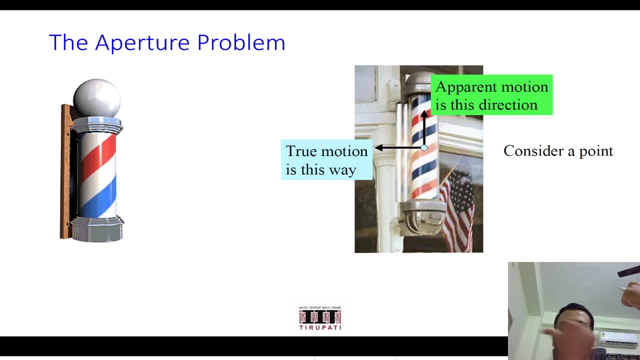 what you would see is, in fact, the true motion is in the parallel direction. so it is rotating in parallel, not in this direction. this is the very common example- here again, this kind of illusion is also coming notice that the gradient is in a skewed direction. it is not. 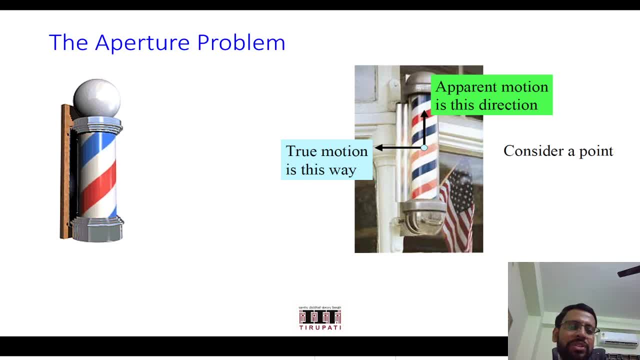 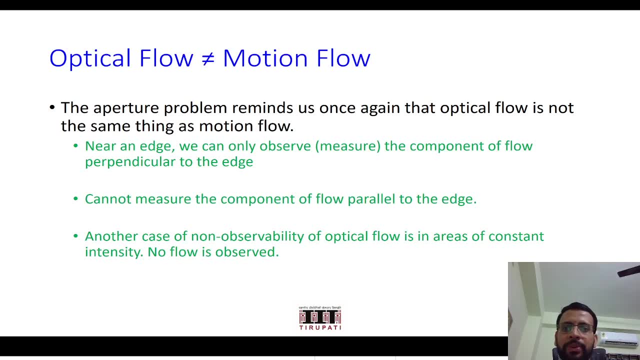 either parallel, vertical or horizontal, so that gives you this effect as well. this is also, in a way, can be attributed to the aperture problem. from the previous illustrations you could see that optical flow is not exactly motion flow. it is because of the aperture problem. sometimes it might not give you exact. 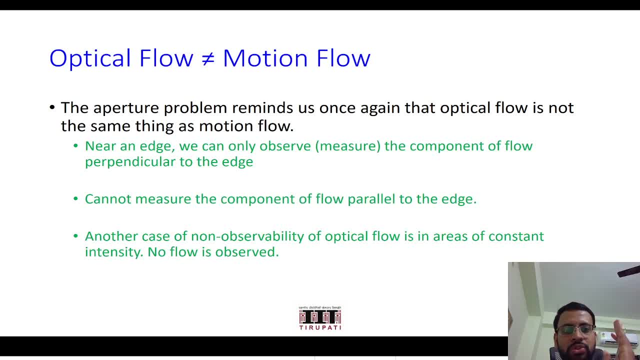 motion of the object so near an edge, you could only observe the component of flow perpendicular to the edge and you cannot measure the component which is parallel to it. okay, also another thing: is suppose, when you this, you have you would have noticed it, even the die that is there, the checkerboard. 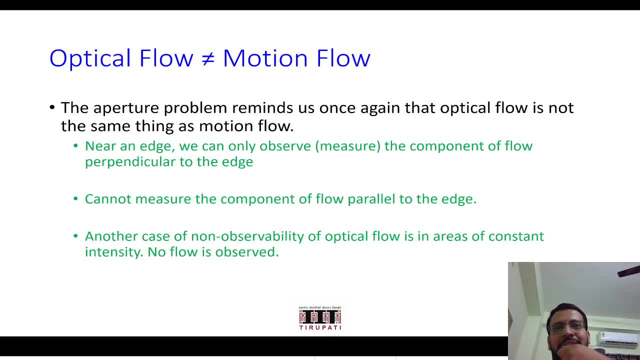 that is there which is rotating on a table in the previous class. there also, you would see where there is a uniform region. you won't be able to see where it has moved because, that being a uniform region, despite, there is a moment at that pixel itself: the. 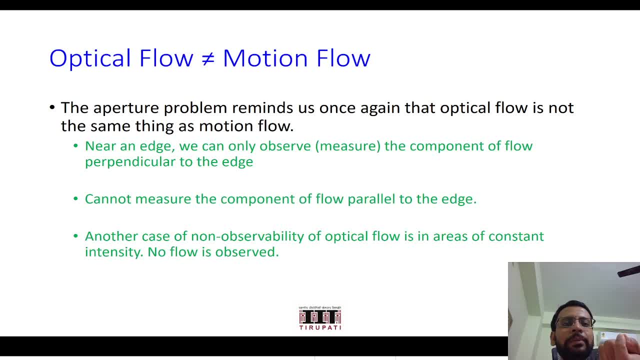 constant intensity is there. all you are looking at the way you are looking at it for its corresponding pixel is that you are looking surrounding it, searching for a pixel that has the same intensity. that being uniform intensity, it could get mapped to any of the those pixels. so 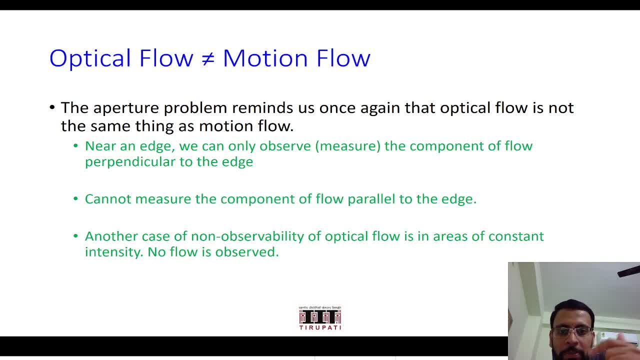 another case of non-observability. so to repeat again, you could observe components that are only perpendicular to the edge, parallel to the edge. you won't be able to do that, and also if the region is uniform, you this will not work out. so you cannot observe really any. 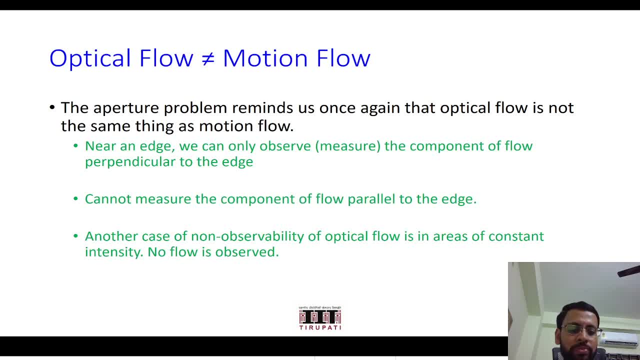 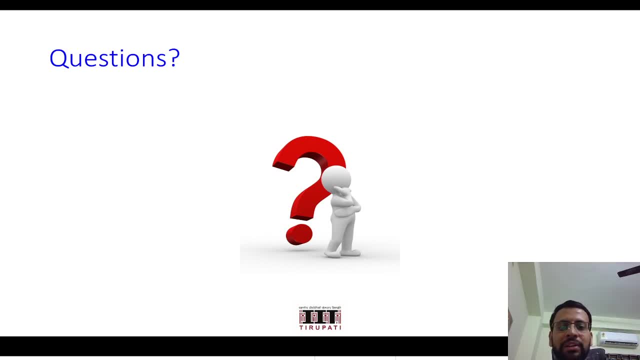 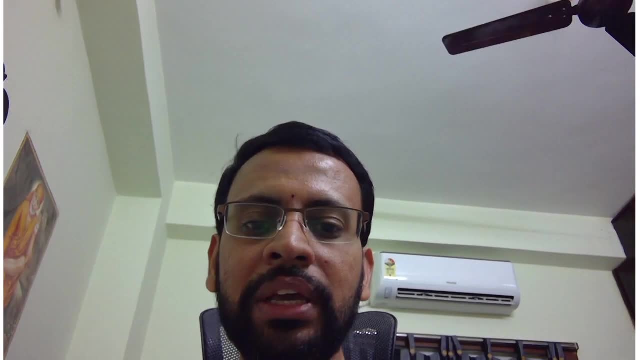 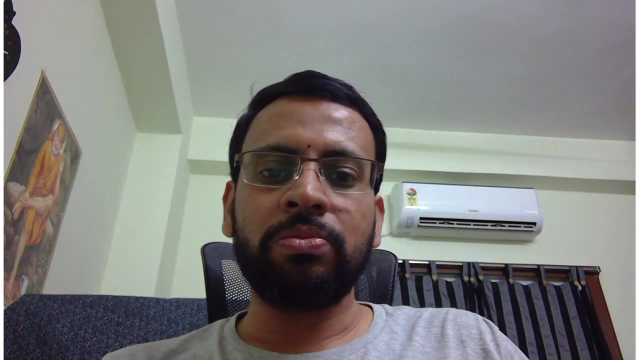 motion flow, despite there being a motion flow. okay, so that's all for this lecture. we just looked at the very basics here in this lecture. so far we posed here only the brightness constancy constraint. in the next lecture we would be imposing few more neighborhood constraints, also assuming 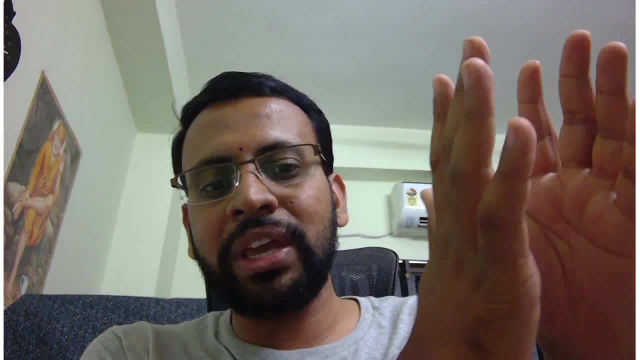 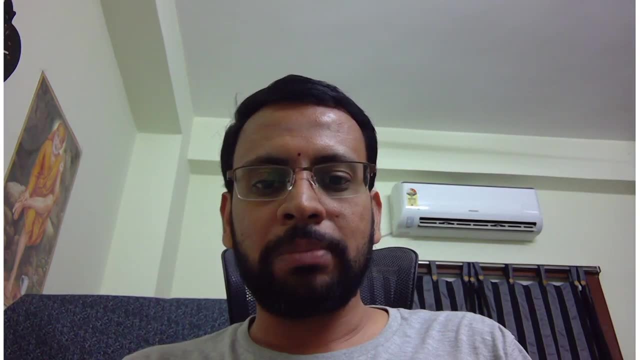 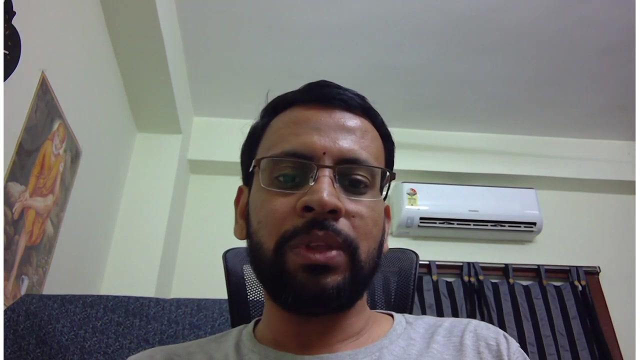 for example, in a motion, all the neighborhood pixels would be moving in the same direction. such constraints will be studying particularly. we will be studying about two specific methods: okay, lokas and canada, horn and shank to begin with, and then we go to lokas and canada method. okay, hope.